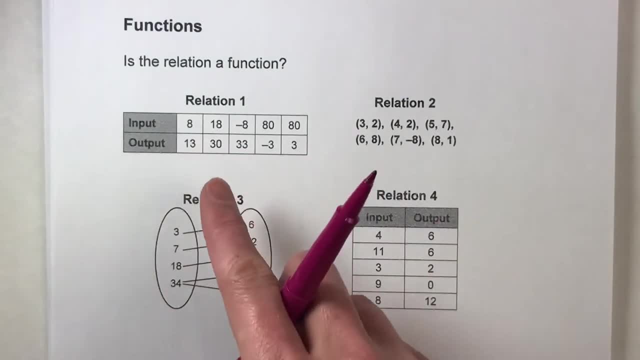 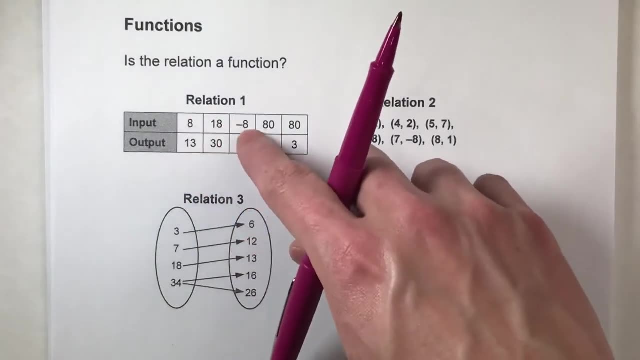 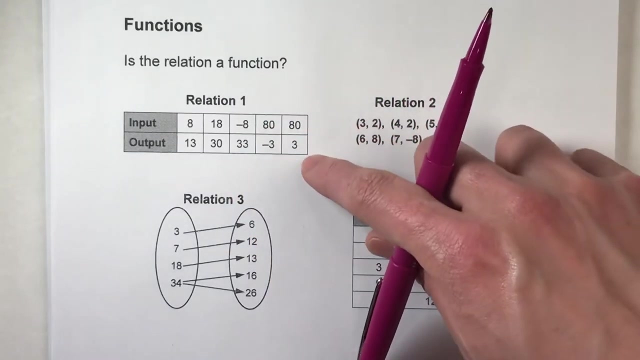 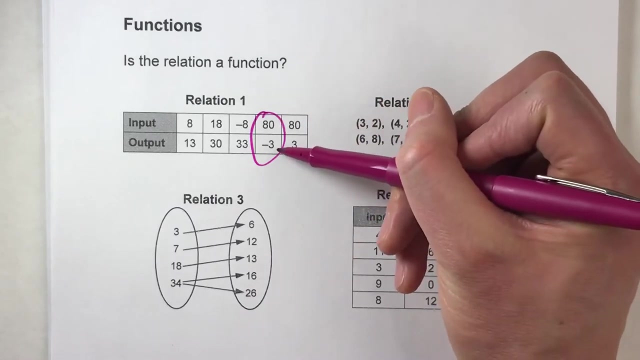 So let's kind of go through these. Relation one: is it a function? Well, an input of eight gave us a 13.. An input of 18 gave us a 30. The input of negative eight gave us a 33.. An input of 80 gave us a negative three, And then an input of 80 again gave us a positive three. Now notice right here: If you input 80 into this relation, I get negative three, And if I input 80 again, I get a positive three. Now that makes this. 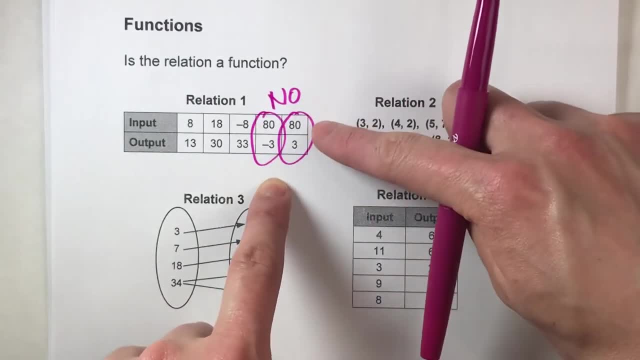 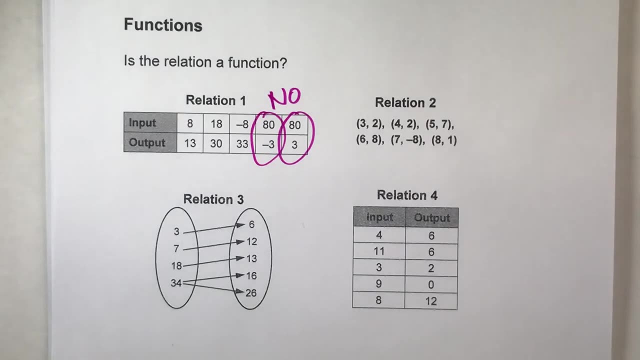 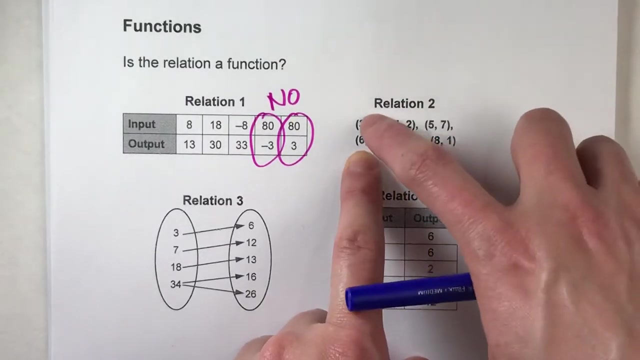 not a function. You can't input the same number into a relation and get two different outputs, All right. So that makes it not a function, All right. Look at relation two. It's very similar, except it's not written in a table format, It's written as a list of coordinates. But you can kind of read it the same way. Three is my input. 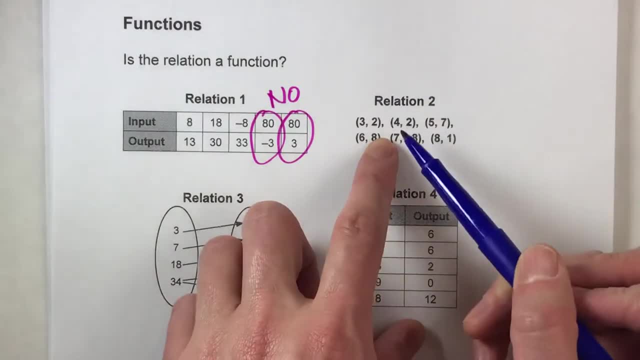 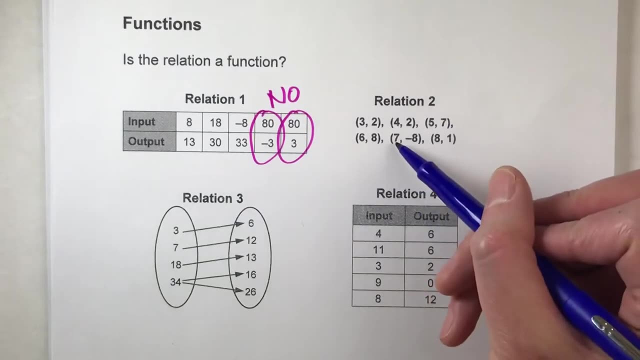 two is my output. So if I input three, I output two. If I input four, I get a two. Input five: 7.. Input 6,, I get an 8.. Input 7,, I get a negative 8.. And I input 8, I get a 1. Notice for every. 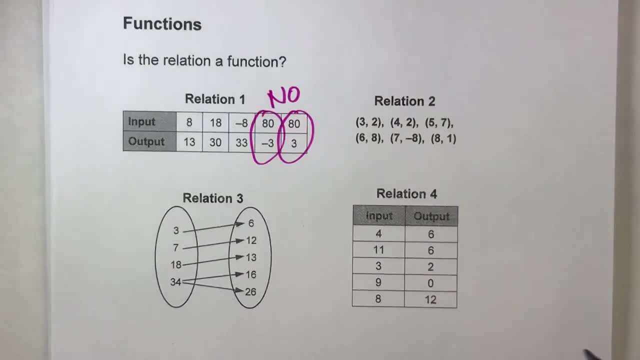 single one of these inputs, I only got one output. This is a function, All right, And again, you don't really have to figure out what the rule is to calculate the output. You're only checking to see if every single input gives us one output And if it doesn't, it's not a function. If it does, 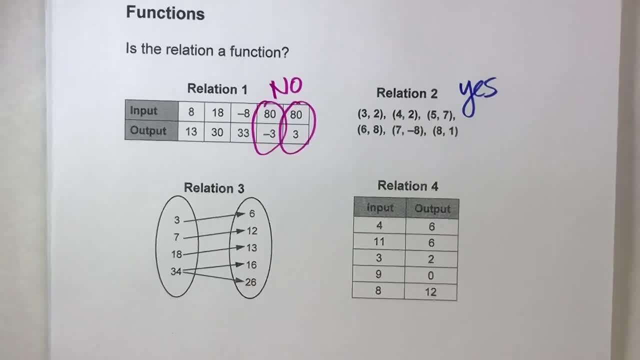 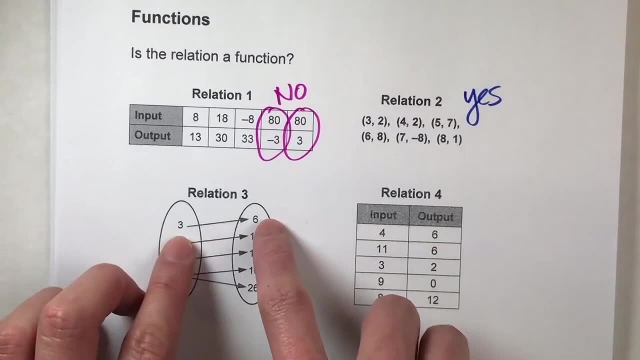 then it is Here. let's do example 3.. So in this example, the arrow diagram, the first set of numbers are your inputs, The second ones are your outputs, And you know that because of the arrow. It's basically saying: my input of 3 gives us an output of 6.. An input of 7 gives us an output of 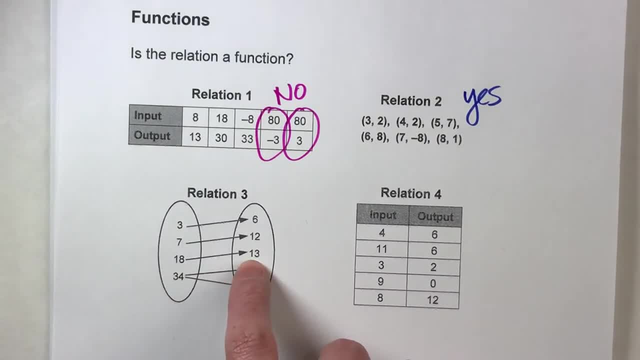 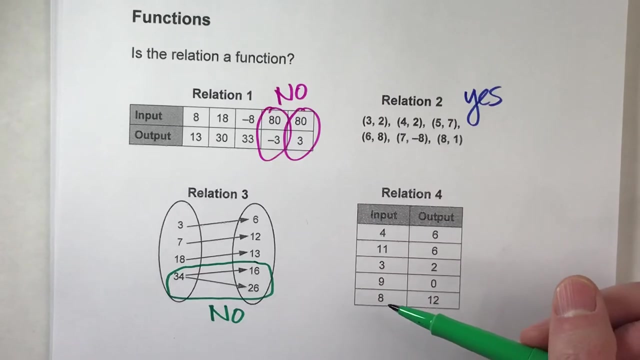 12.. The input of 18 gives us an output of 13.. And then the input of 34 gives us both 16 and 26.. So you could see right away this one right here. this makes this not a function, because an input of 34 gave us two different.